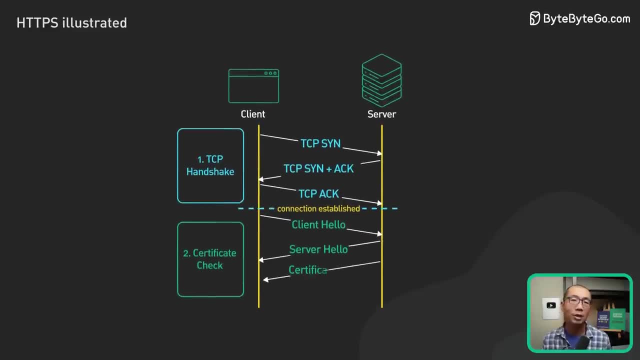 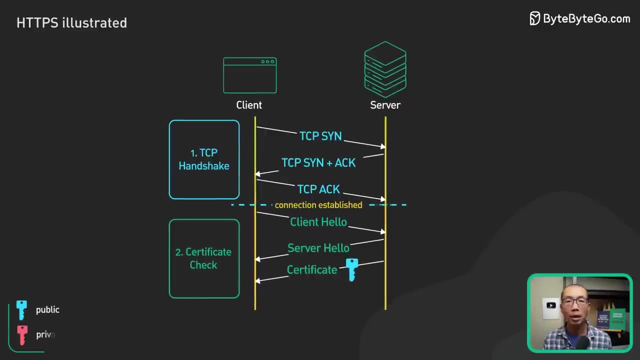 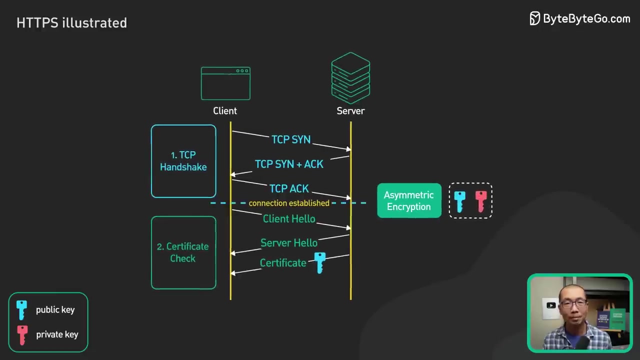 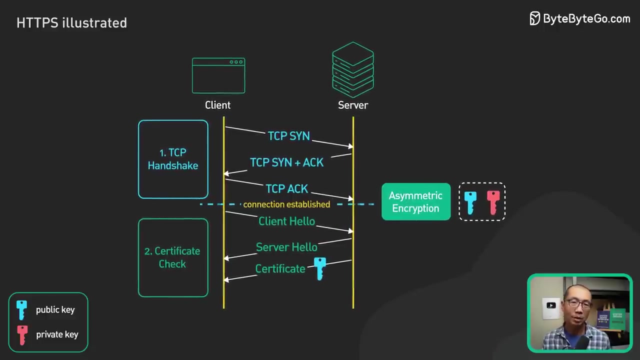 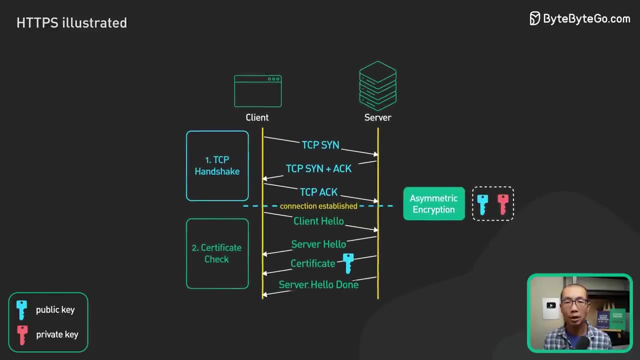 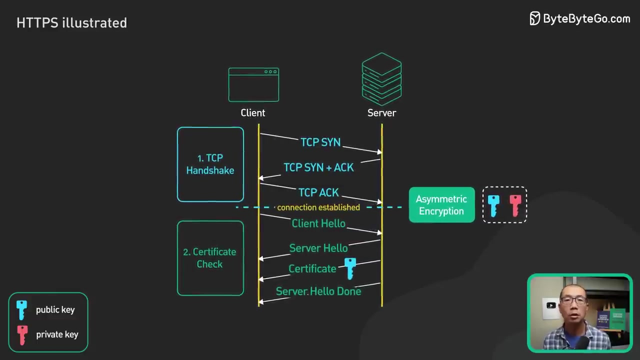 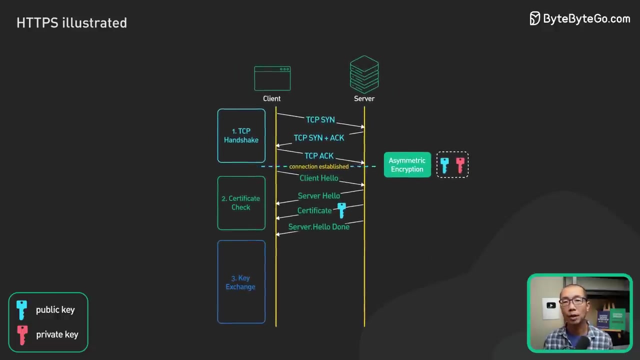 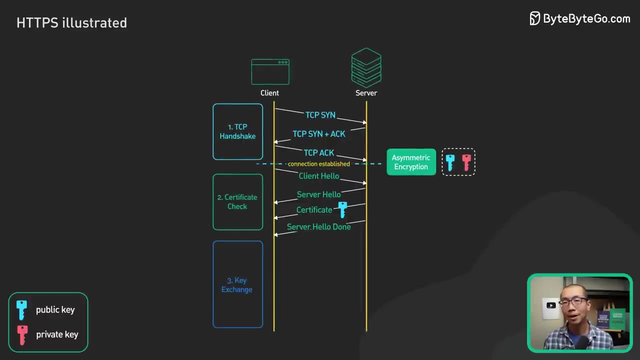 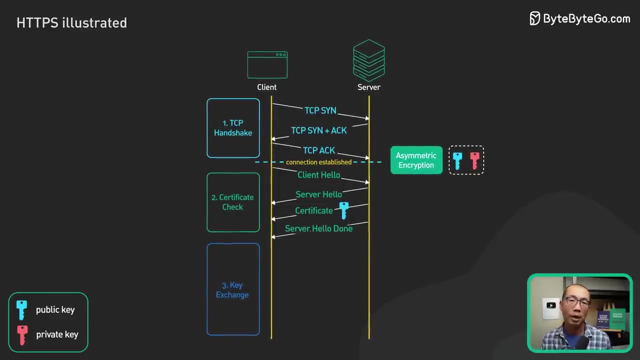 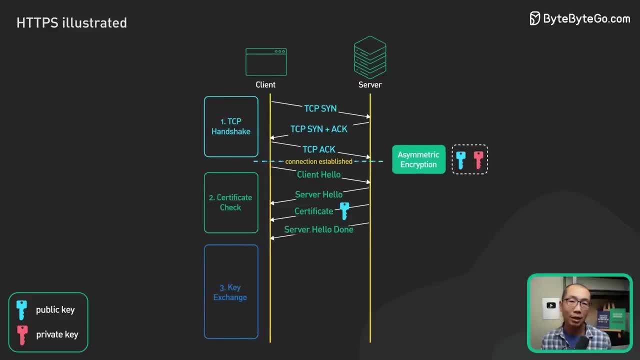 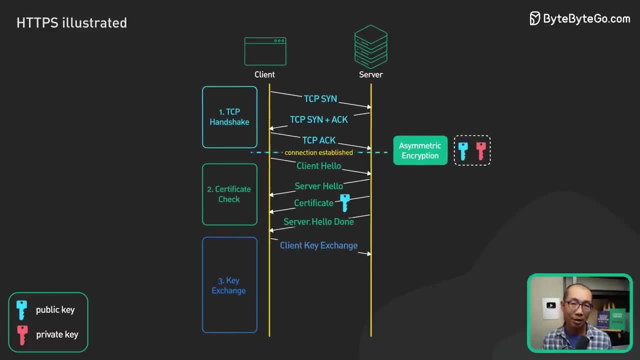 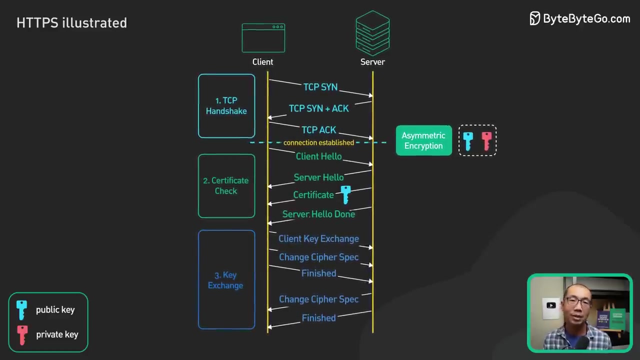 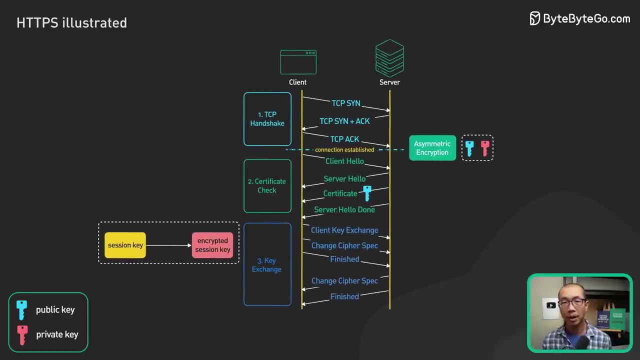 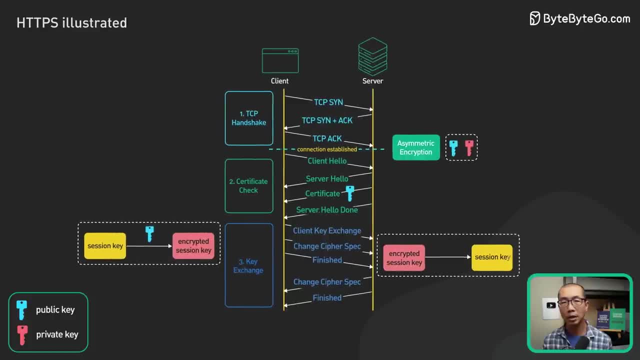 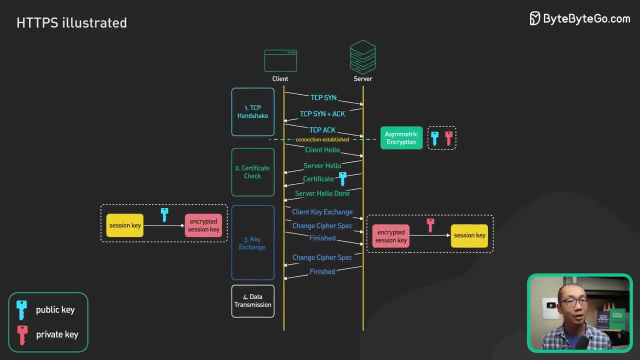 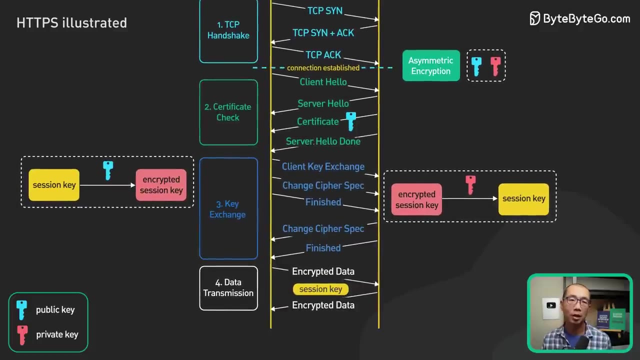 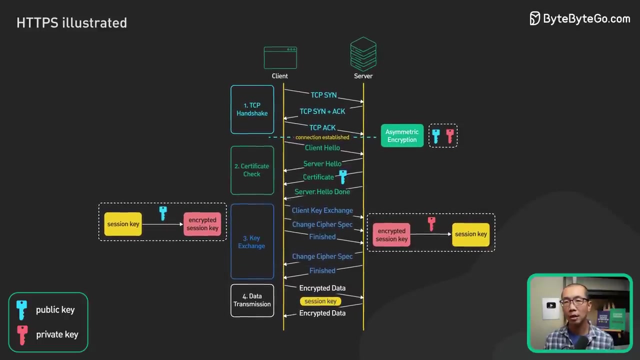 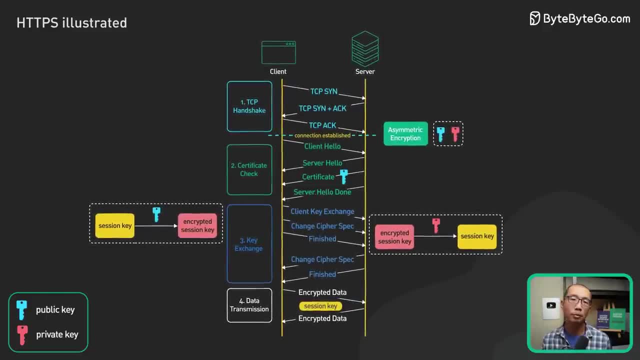 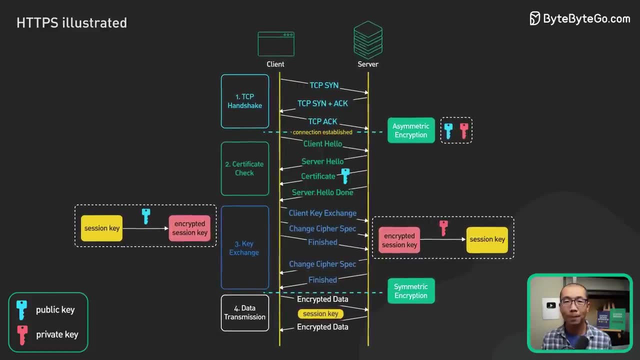 computationally expensive. It is not really suitable for bulk data transmission. Before we close, there are two final points I would like to discuss. First, the handshake we talked about applied to TLS 1.2,, while the latest version is TLS 1.3,.